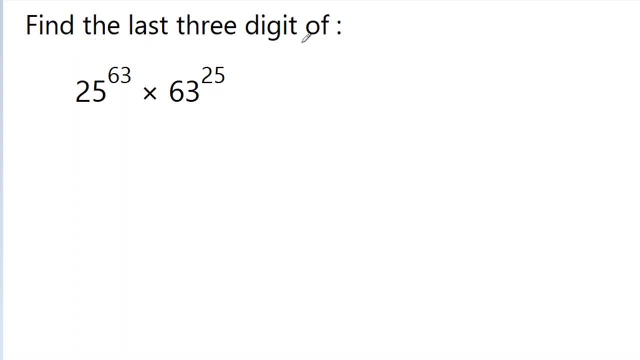 In this video we have to find the last 3 digits of 25 to the power 63 into 63 to the power 25.. So calculating it manually is not possible. So here the logic I am going to use is: if we have any number- suppose 1692- and if we divide this number by 10, then we: 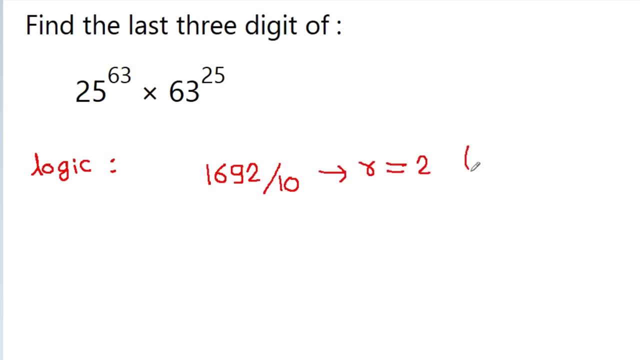 get remainder equal to 2.. That is the last digit. and if we divide this number- 1692- by 100, then we get remainder equal to 92.. That is I last 2 digit. and similarly, if we divide this number by 1000, then we get remainder equal. 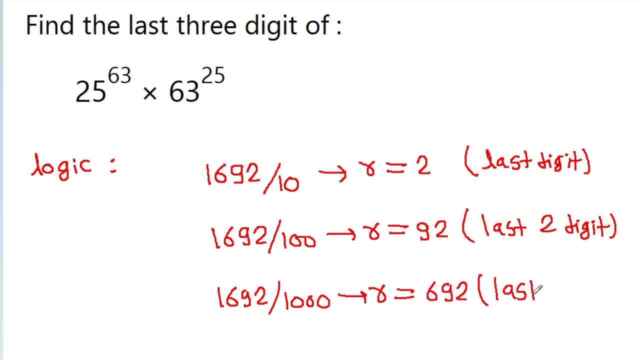 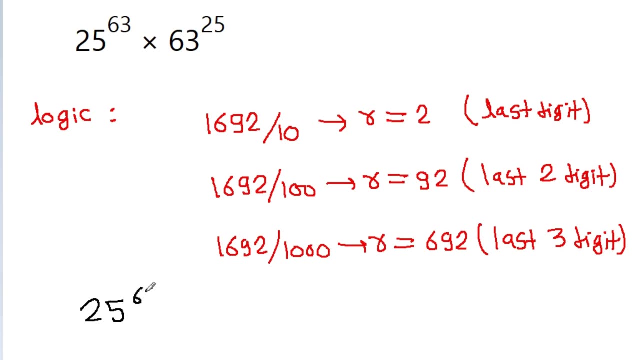 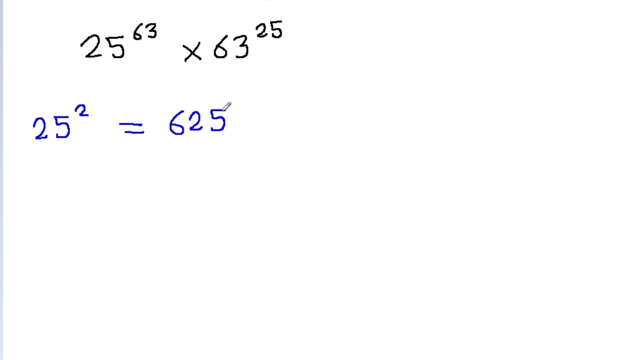 to 692. that is last 3 digit. so I am going to use this logic in this problem. so here we have 25 to the power 63, into 63 to the power 25, and now if we focus 25 to the power 63, then 25 square is 625 and 25 cube will be 25.. 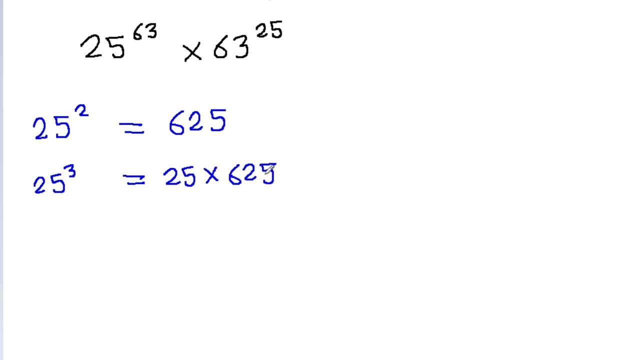 25 into 625 and multiply any number by 25 is easy. just multiply the number by 100 and divide it by 4, then we get 15625, and this can be written as 1000 times some constant k2.. So this is our solution. 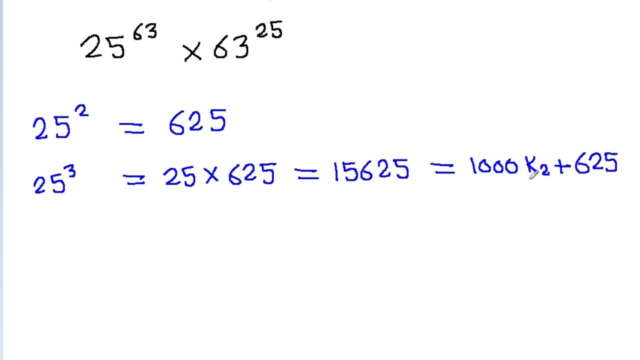 K2 plus 625, where k2 is 15, and this can be written as 1000 times some constant k1 plus 625, where k1 is equal to 0. Now if we try to calculate 25 to the power 4, then that will be 25 times 25 cube that. 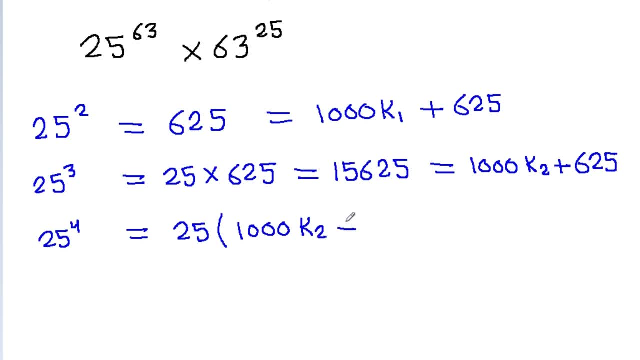 is 1000 k2 plus 625. And then this shows us that is 4000k2 plus 625percent times k2 is 15625.. So this is our solution, And here also we can write this as 1000 times 625. here k3 is aside from k2 and below k3. 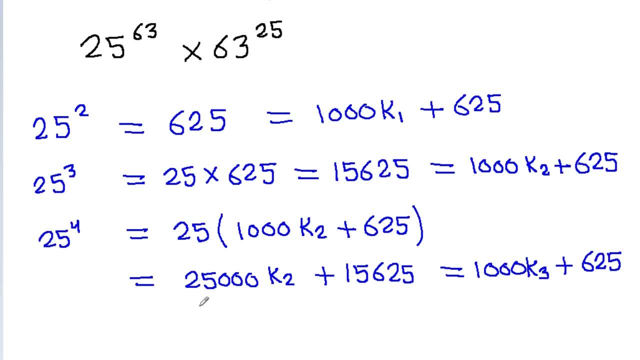 it is 12 awful times laws, k2 extra and 5 times 625. So we have 15.. Or binahere, we have 15.. This is our solution: Travis separated by 0.. By following the pattern, we can write 25 to the power 63 as 1000 times some constant. 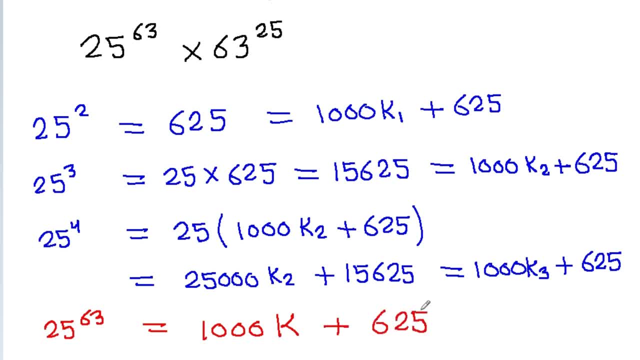 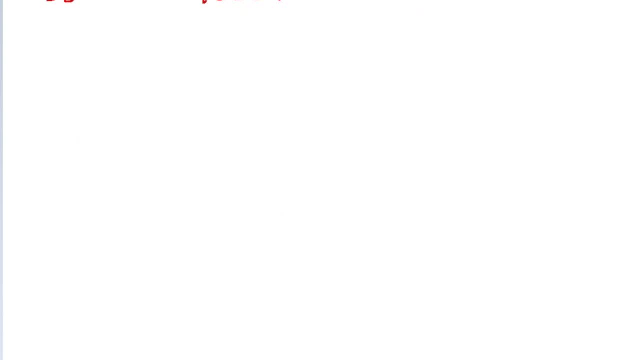 k plus 625. and now if we focus 63 to the power 25, then 63 is close to 64. so we can write this as 64 minus 1, or it can be written as 8 times some constant c1 minus 1, and now 63. 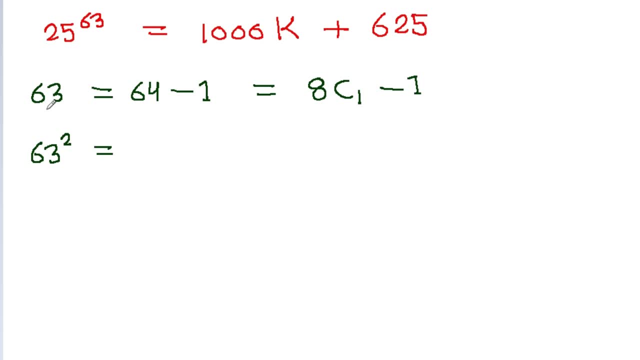 square can be written as 63 into 63, that will be 8c1 minus 1 times 8c1 minus 1, and now we here: hc1 into hc1 is multiple of 8, and hc1 times minus 1 is also multiple of 8 and minus. 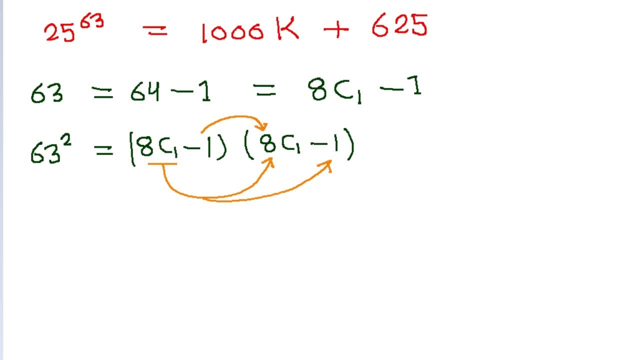 1 times hc1 is also multiple of 8.. So the only minus 1 times minus 1 is not multiple of 8.. So we can write this as: 8 times some constant c2 and minus 1 times minus 1 will. 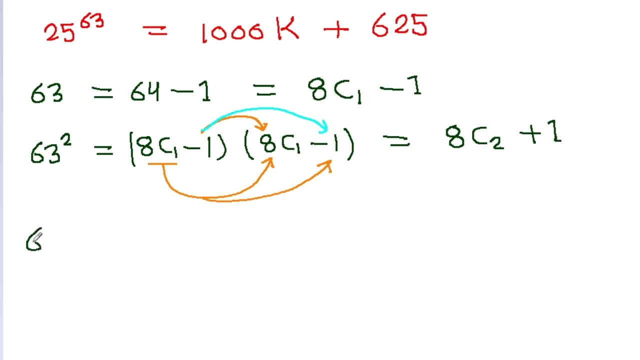 be plus 1, and now 63 cube can be written as 63 into 63 square. that will be 8c1 minus 1 times 8c2 plus 1, and here also everything is multiple of 8 except this minus 1 times. 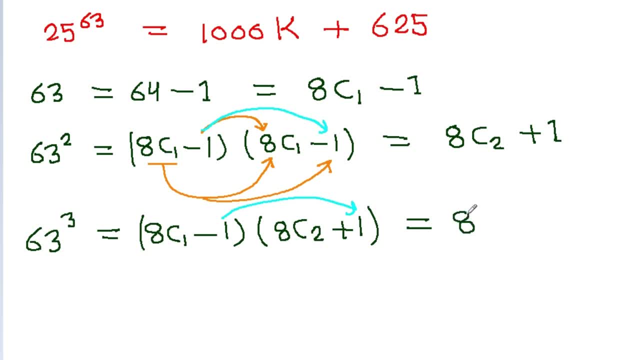 1.. So we can write this as 8 times some constant c3 and minus 1 times minus 1.. and minus 1 into plus 1 will be minus 1. so by following the same pattern we get 63 to the power. 25 is equal to 8 times some constant C and here in even power we have plus 1 and 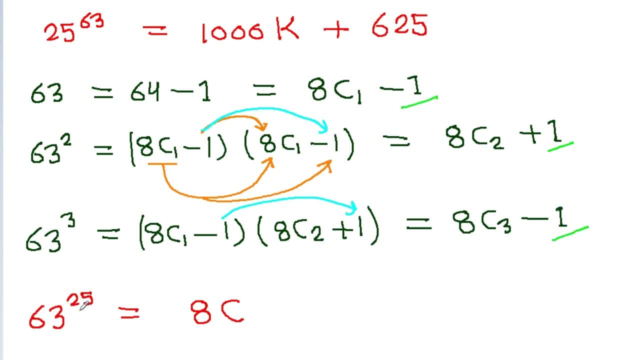 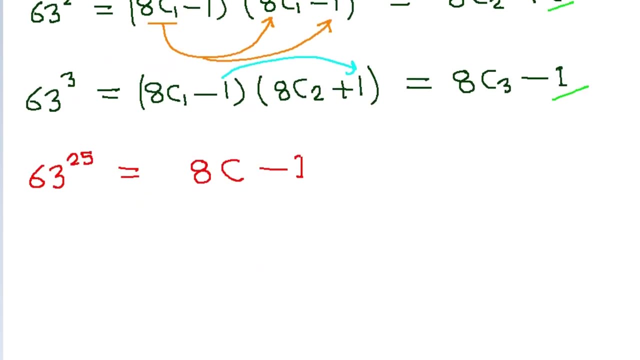 in odd power. we have minus 1, and 25 is odd, so we get minus 1. now we have to find the last three digits of 25 to the power 63 into, 63 to the power 25, so 25 to the power 63 into. 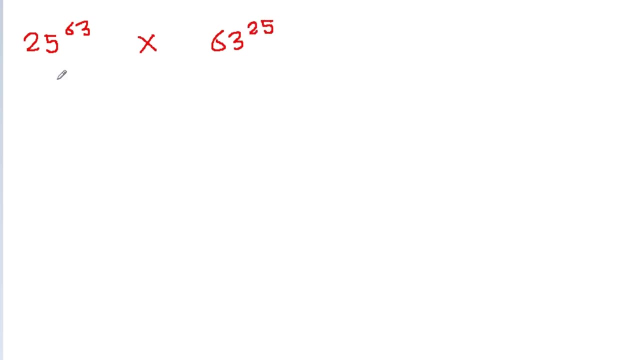 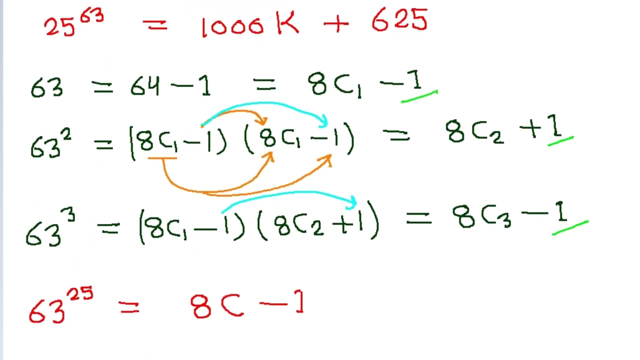 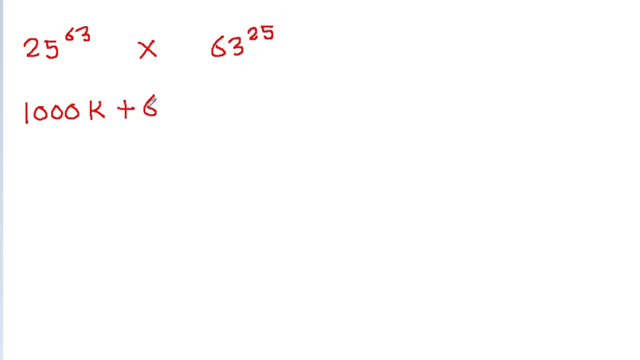 63 to the power 25 will be 25 to the power 63.. 63 is 1000 K plus 625. it can be written as 1000 K plus 625, and 63 to the power 25 can be written as 8 times C minus 1, 8 times C minus 1. and now if we multiply it, we get 63. 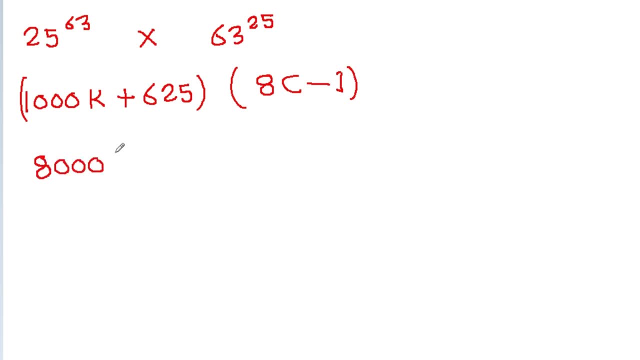 to the power 22, we get 8000 times KC minus 1000 times K plus 625 into 8 will be 5000 times C and minus 625. or we can write this as 8000 KC minus 1000 K minus 625 and we get: 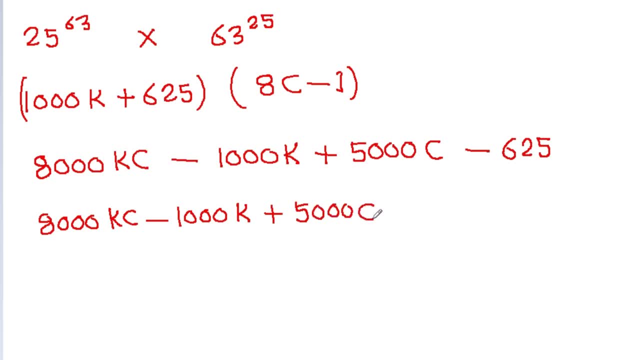 8000 times K C minus 1000 times K plus 625, and we can write this as 8000 times K C minus plus 5000 C and minus 625 can be written as minus 1000 plus 375. and now these: